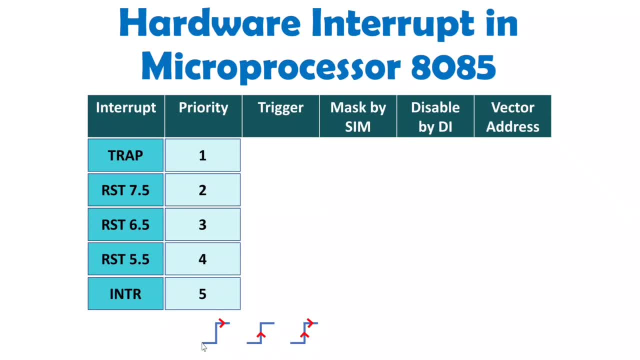 you can observe. but if you observe here, when signal is going low to high and when it remains high, at that time here arrow is indicated. so arrow indicates what? arrow indicates triggering location. so whenever you have arrow with this logic high, which is remaining continuously over here, what it means this is level trigger. the reason is: whenever it is having logic. 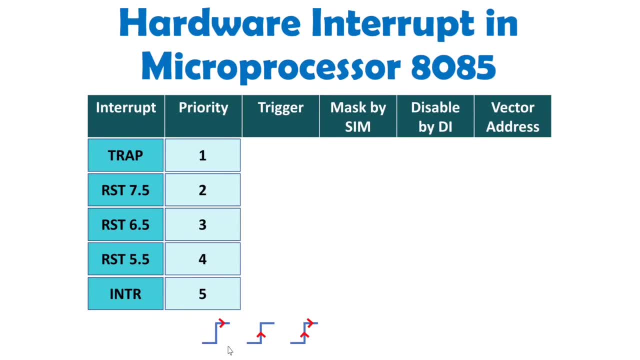 one, it is having level trigger and when it is having level trigger it is having level one. at that time it will get trigger. so this is level trigger signal. when it comes to age trigger, at that time, you see, whenever there is a transition from low to high, at that time there. 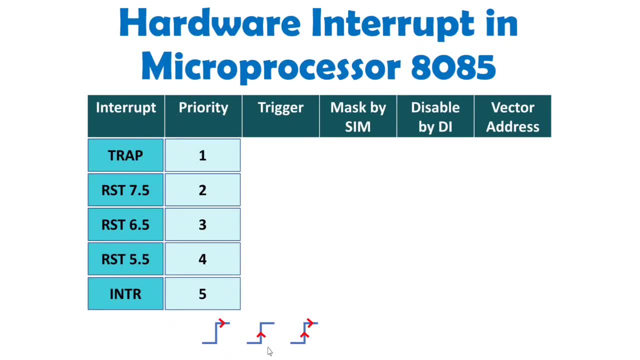 is a triggering. so this is age trigger and you see, here we have transition from low to high. at that time also there is a triggering. and whenever it is remaining high, at that time also there is a triggering means this signal that indicates your interrupt is level as well as age trigger. 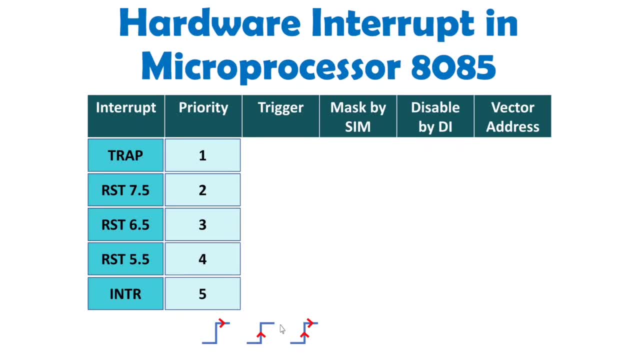 now, my dear students, there are some basic things that you must know. see, trap is having highest priority, so trap should get trigger with age as well as level. so you see, with trap we have age as well as level triggering right. the reason is in age as well as level. we have age as well as level. 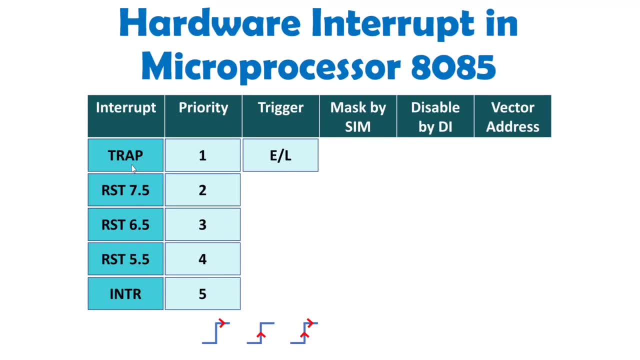 in any situation, this trap should have service. i'll explain you some examples. even right now, just consider: this trap should have services with age trigger as well as level trigger. now, with microprocessor 8085, there is only one interrupt, which is age trigger. that is rst 7.5. so rst 7.5. 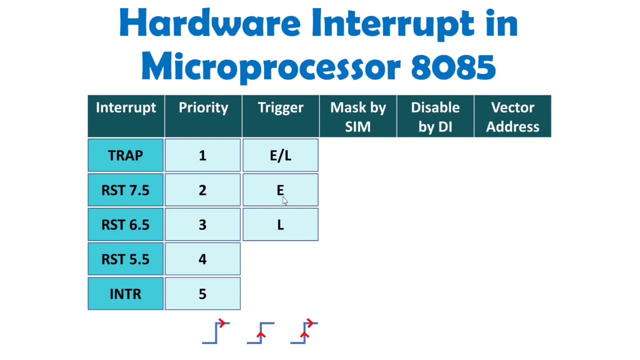 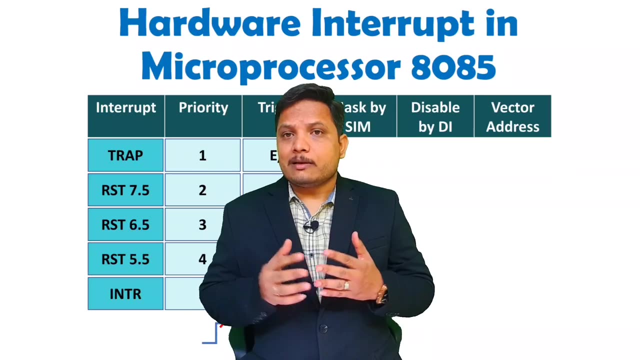 that is only age trigger. and rst: 6.5, 5.5 and intr. those are level trigger. now, my dear students, let me explain you some practical cases so that will get more clear students, let me give you one practical example. what is the meaning of age? 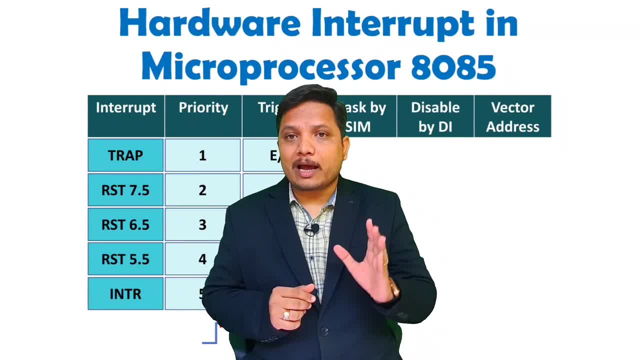 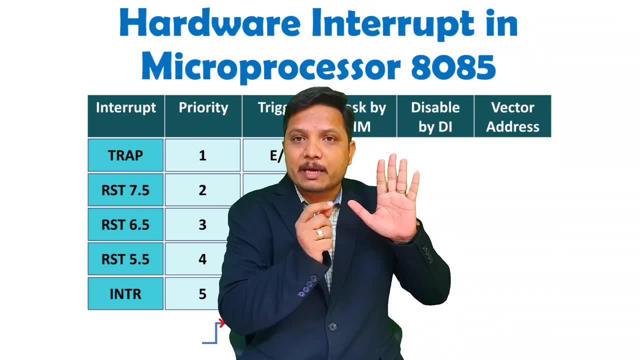 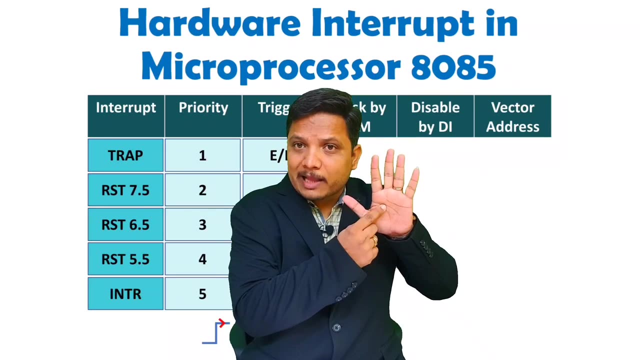 trigger. see, for example, you are having your mobile in which you just press one button. let us say, you are typing something and you are pressing key a. so when you press key a, what will happen? it will display a right. if you continuously press key a, is it like it will be pressing a, a, a, a a like this? no right. so what? it means this. 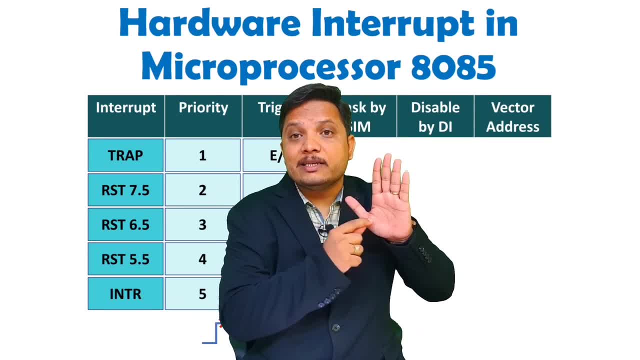 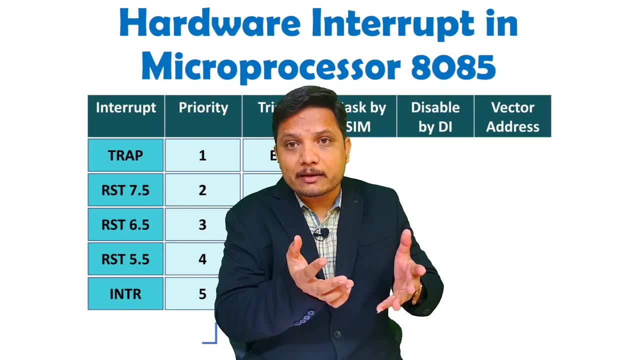 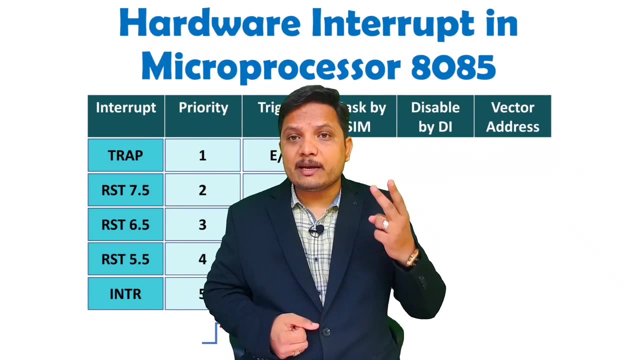 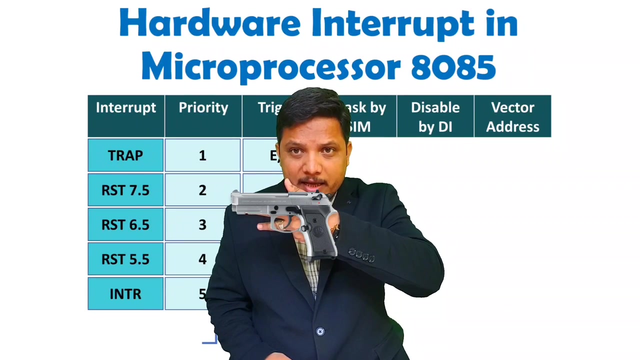 pressing of key. that is age trigger. but when you continuously press something and if it is responding to that, what it means it is level trigger. let me give you one practical example again. see, you are having a revolver now you just shoot that by having a trigger. so here I am having a trigger right now. when I press this trigger, what will? 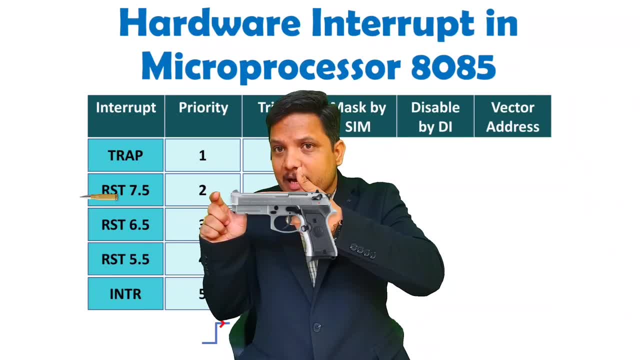 happen from the nozzle, it will fire a bullet. right now. if I want to fire second bullet, what I need to do I need to release this trigger and then again I To press to have second bullet right. So this is how edge trigger pistol is there. 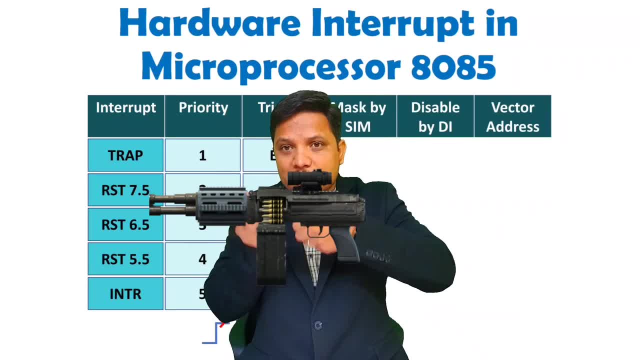 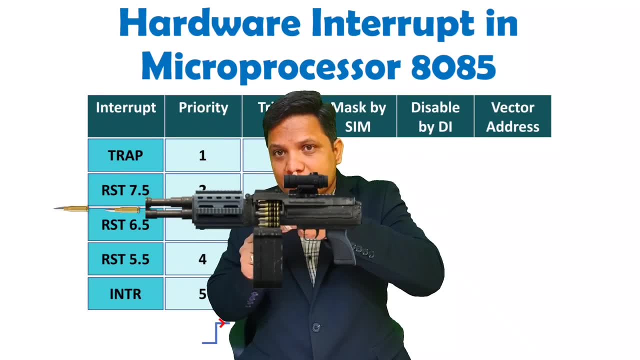 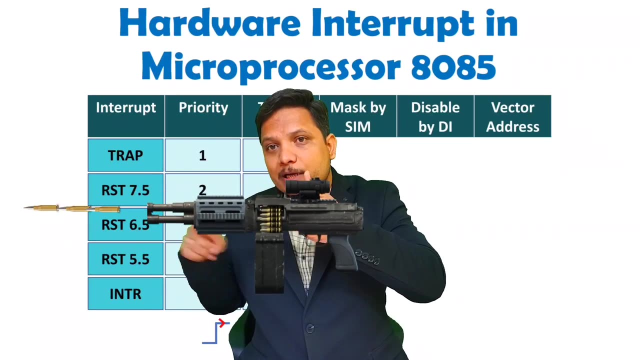 But let us have machine gun. So in machine gun, let us press switch Means, let us press trigger. When you press trigger, what will happen? Machine gun will continuously firing bullets. It will continuously fire bullets. You don't need to release this. 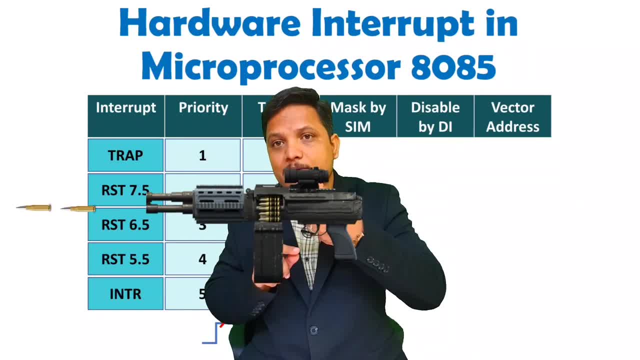 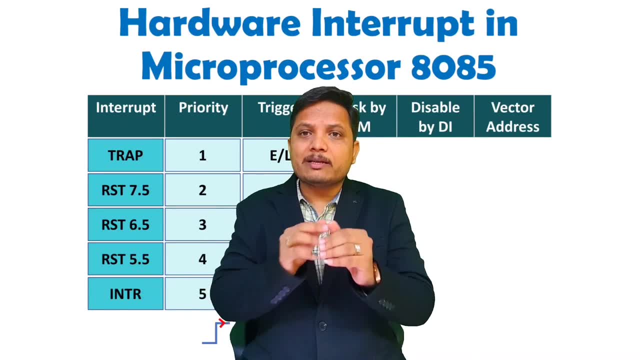 You just press it right, It will continuously fire bullets. So what is the meaning of it? It is level trigger. So, my dear students, edge trigger means what? Whenever there is a transition from low to high, at that time it should get trigger. 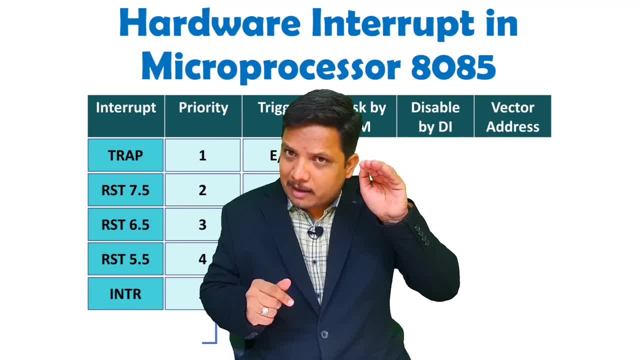 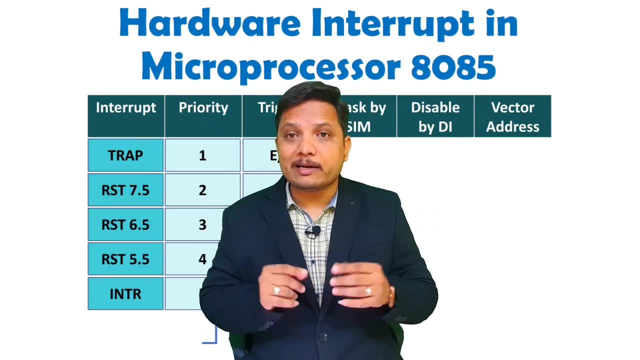 And level trigger means what: It should remain high for some time period to get recognized. That is how it is there, right? So microprocessor is having trap, that is, edge as well as level trigger, And with microprocessor only 7.. 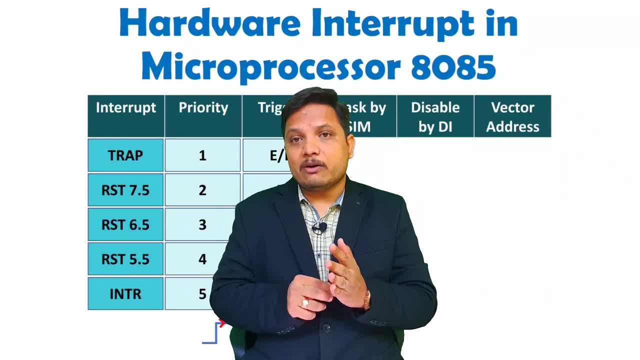 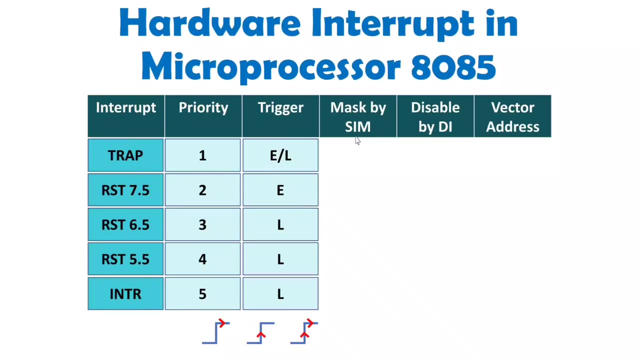 RST 7. 5,, that is having facility of edge trigger, rest. RST 6. 5,, 5.5 and INTR, those are level trigger. Now when we talk about mask by SIM then you should know in SIM instruction you can mask. 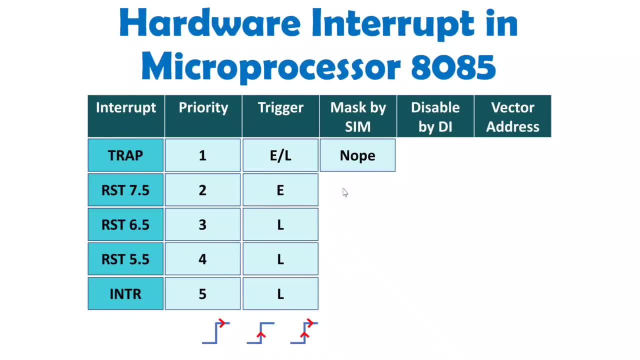 RST 7., 5,, 6. 5 and 5.5.. So trap and INTR that cannot be masked right. So you should know this, my dear students: In SIM instruction: we can mask RST. 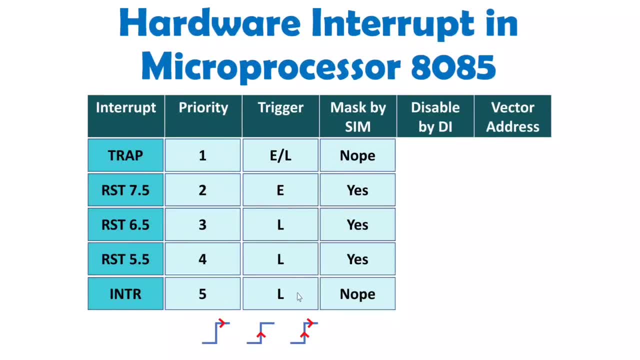 7., 5,, 6., 5 and 5.5. INTR and trap cannot be masked. Now when we talk about, can we disable these interrupts? So only trap cannot be disabled. right, It is having highest priority. 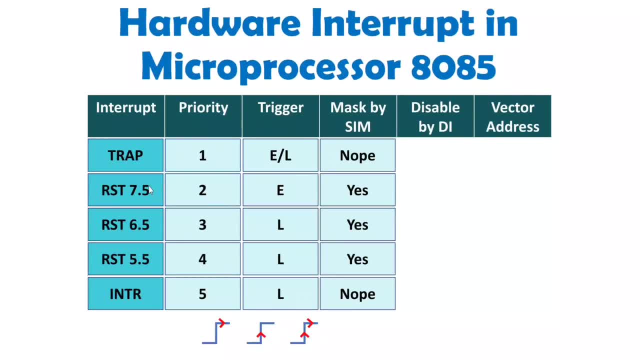 So you cannot disable this trap. Rest of these interrupts can be disabled. right Now let us talk about how vector addresses are there. So, my dear students, When we talk about trap, then initially its name was RST 4.5 and based on that, we can. 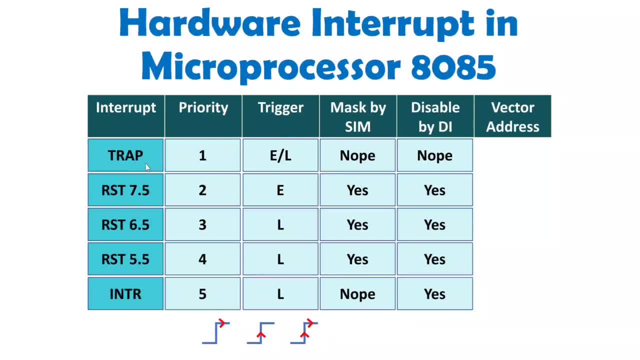 remember its address: 4.5 into 8, that will be 36, and in terms of hacks, it will be 0024 hacks. RST 7.5 address. that is also based on that: only 7.5 into 8 and in terms of hacks, it is: 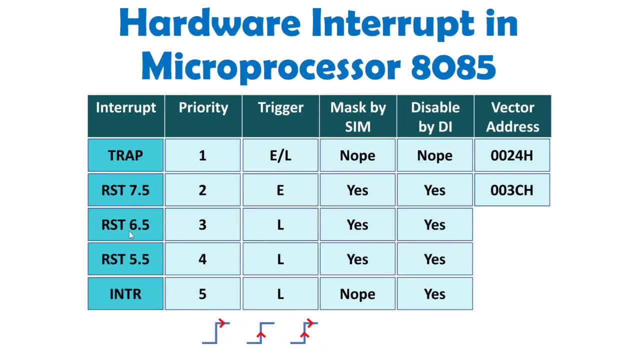 003C hacks, RST 6.5 also there as per 6.5.. Similarly, RST 5.5 into 8, that is, in terms of hexadecimal. it will be 002C hacks and INTR does not have any vector. 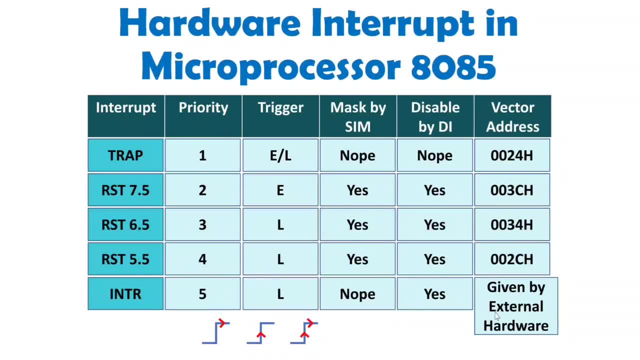 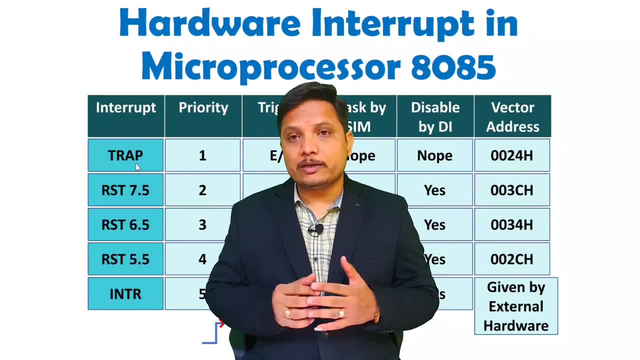 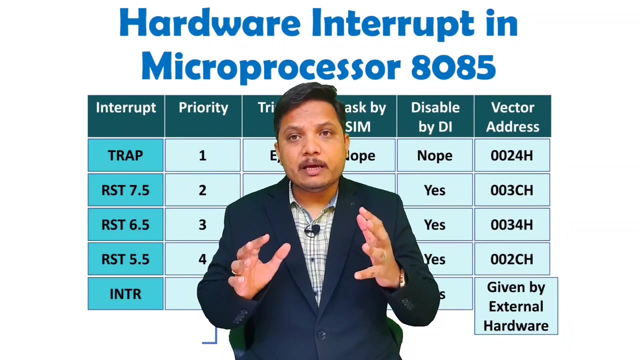 It will be having address as per the instruction given by external hardware. Now, my dear students, you should know some basics like trap. Trap is having highest priority and which kind of operation that we need to perform by trap. So, my dear students, trap is having highest priority and with trap we will be interfacing. 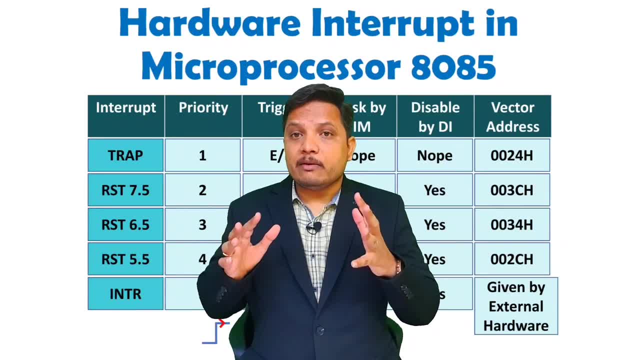 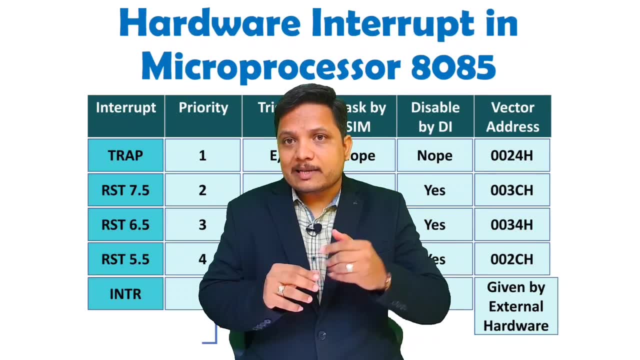 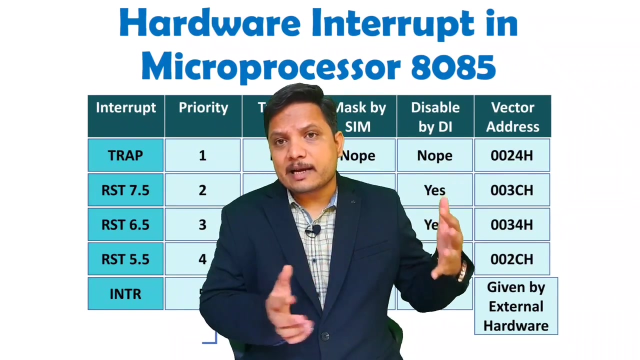 those devices which are having very essential work, Like, for example, you are having a car and this car is having many other interrupts, like AC temperature, Like door lock, like you may be having music player, like you may be having light interfacing inside for interior. 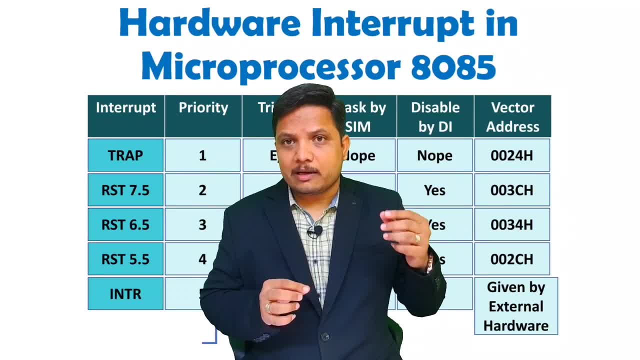 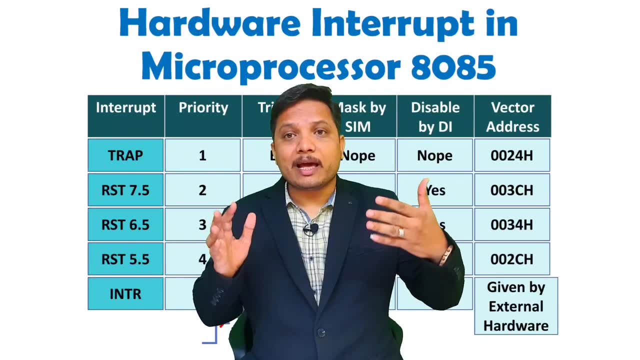 So there are many interrupts which is there inside of car, But with trap kind of interrupt you should be providing very essential work, Like whenever accident is coming. at that time there cannot be delay, It should be having highest priority and it should give. 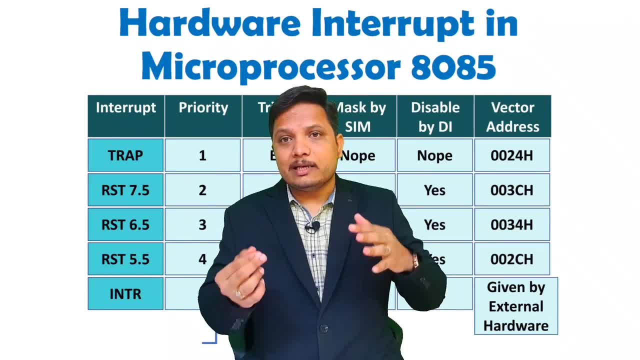 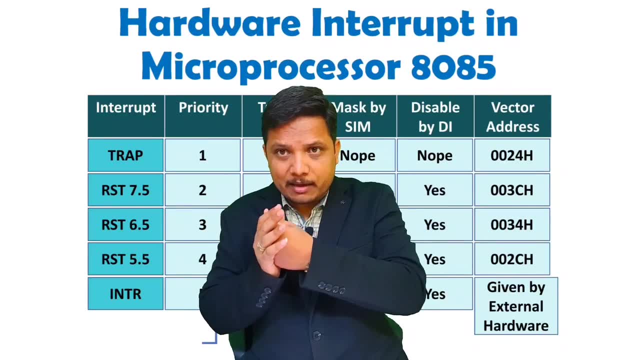 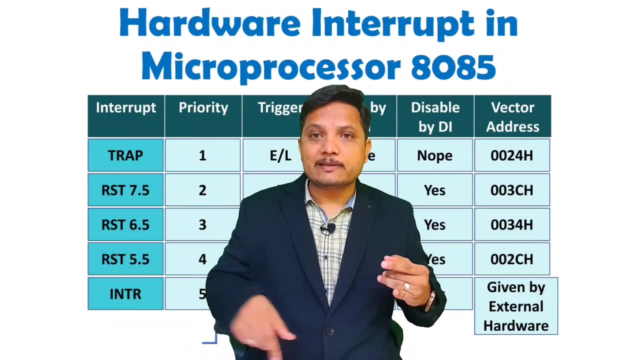 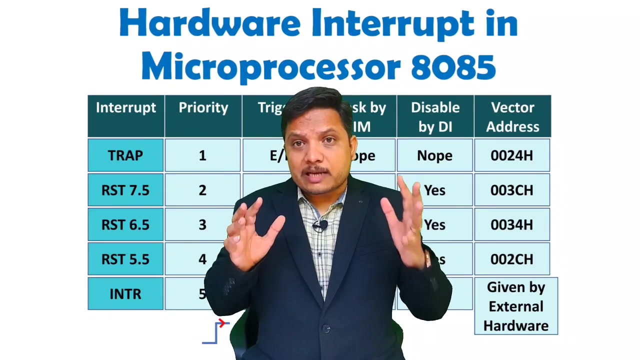 Service immediately. So for that, inside balloon should get opened up immediately whenever accident is coming. Right, So whenever car is having accident, at that time immediately there should be opening of balloon inside so that people cannot have maximum damage. Right So this type of services that is having highest priority, in which you cannot have any delay. 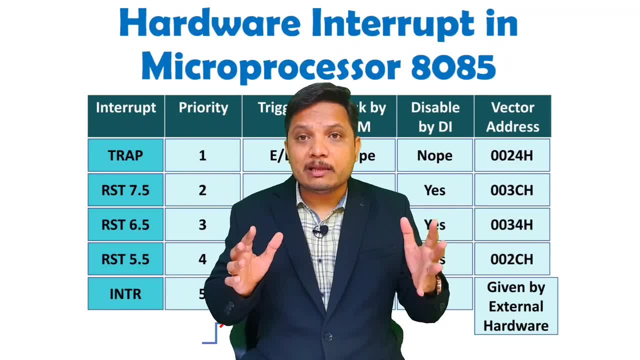 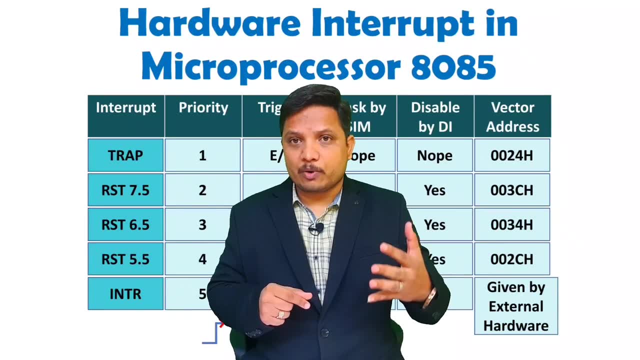 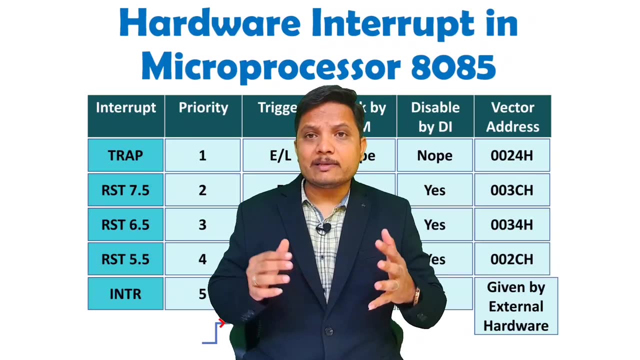 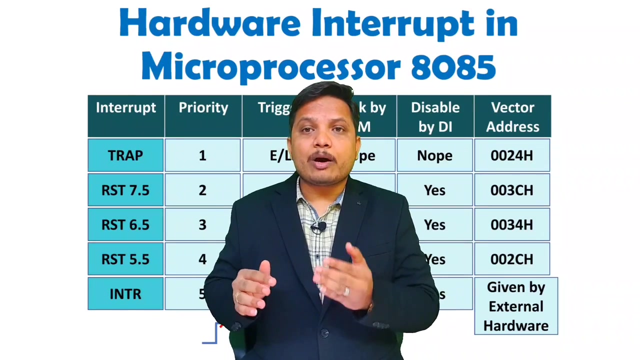 That's why with trap we don't have disable kind of operation right. Disable interrupt cannot even disable trap in between of program. It will get executed immediately, even if anything is happening with microprocessor. So likewise if you talk about mechanical refineries, in that if you are having a boiler 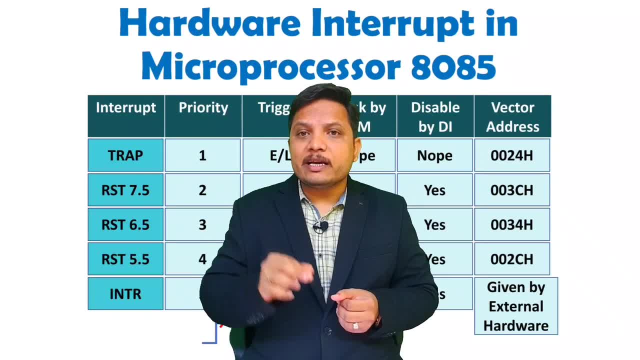 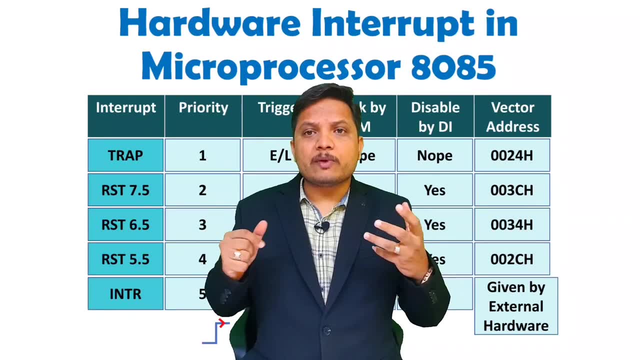 temperature which is having threshold limit of 120 degree of Celsius, And if it is reaching towards 120 degree Celsius of temperature, at that time you should not wait Right. Immediately. it should shut down that boiler so that that temperature cannot rise beyond. 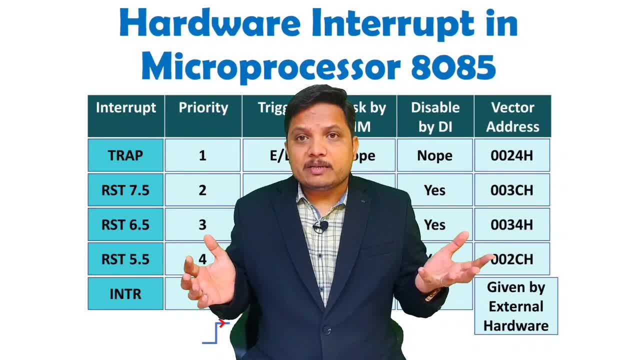 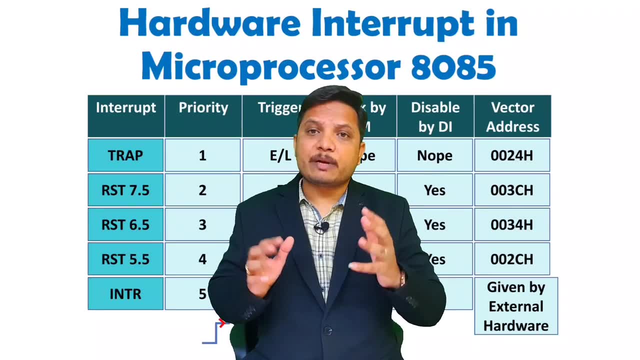 the threshold, Otherwise there can be maximum damage which is possible inside the refinery. So this type of operations, those are being performed with highest priority, interrupt and practically here with this 8085.. It is trap With other microprocessor and microcontroller it is having different names, like with 8086. 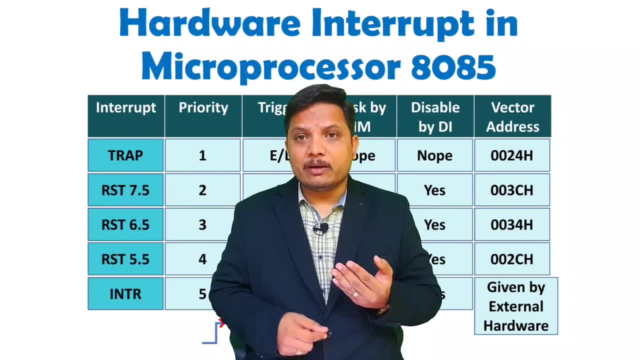 We have an MI non maskable interrupt, right? So you should know, always there will be one interrupt which is assigned with microprocessor or microcontroller that is having highest priority and that will get executed, no matters What does that microprocessor or microcontroller is doing right now.